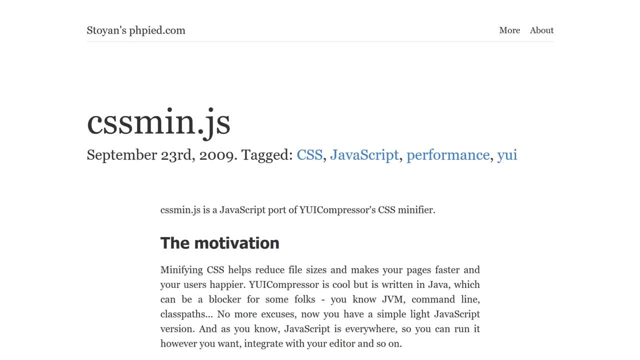 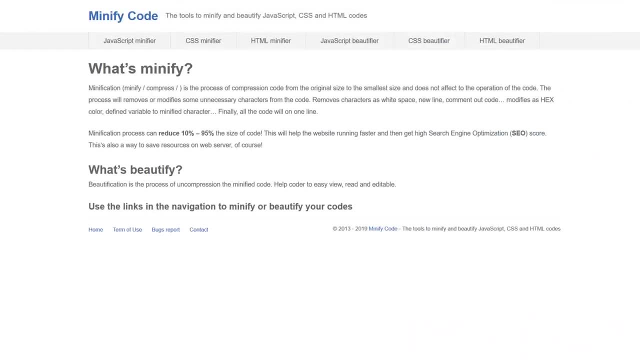 checking out the blog post in the description. If you're looking for some offline tools to minify your code locally, you can use CSSminjs or YUICompressor. Many of the online tools have a similar process and for this example, I'm going to use the minify tools from minifycodecom. 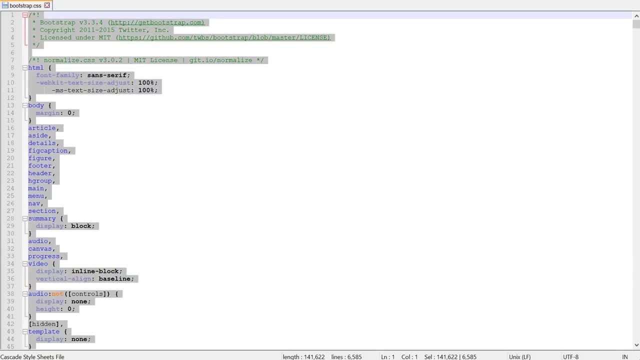 First we're going to click the CSS minifier tab. Then we're going to take all of my CSS code and paste it in. Now we just click minify CSS and there we go. Now we can just copy this code. 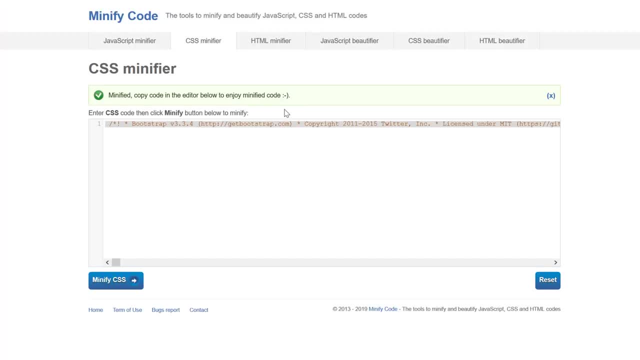 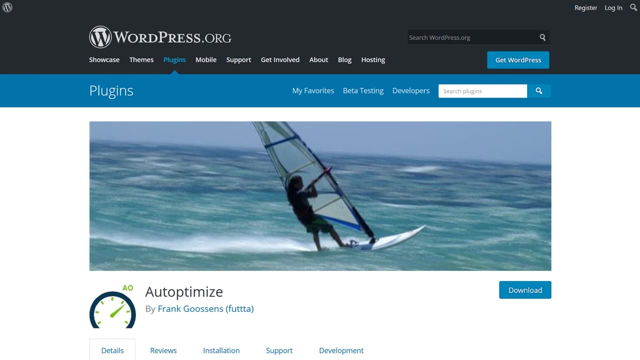 and replace it in my original file. Now you would repeat the same process to minify your JavaScript or HTML files. Now let's talk about how to do this in WordPress using plugins. The first plugin is AutoOptimize, and this is free. It's probably one of the most popular minify plugins out there. 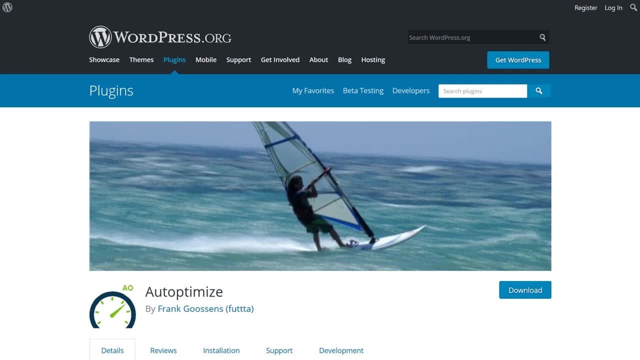 and it's popular because it's easy to use and full of powerful performance features. It can aggregate, minify and cache your code. As a bonus, you have additional options for optimizing Google Fonts, images and more To use AutoOptimize download, install and activate the. 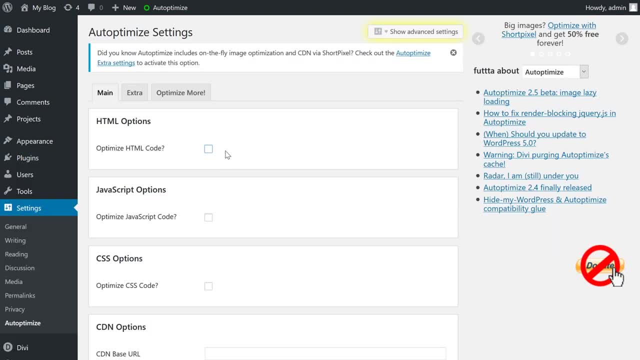 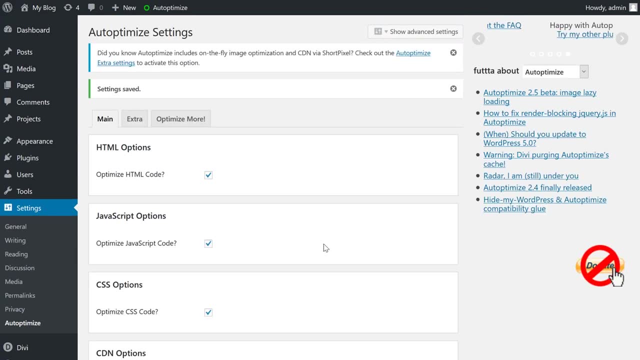 plugin and then navigate to Settings- AutoOptimize. Now we just choose which code we want to be optimized, and then we just have to click Save Changes and we're all set. As you can see, it's pretty simple and very powerful. There are other free WordPress plugin. 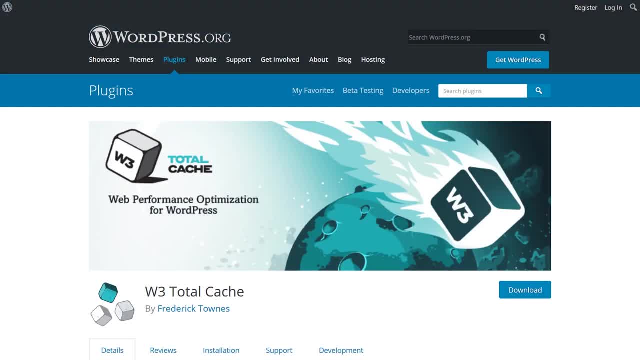 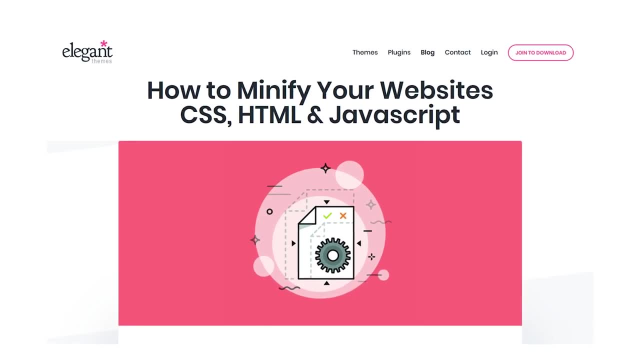 options, and that includes Fast Velocity Minify, W3 Total Cache and WP Fastest Cache, And just like that, you're now a master at minifying your website's files. If this video helped you, then be sure to give it a like and subscribe for more content With that. said thanks for watching and we'll see you in the next one. 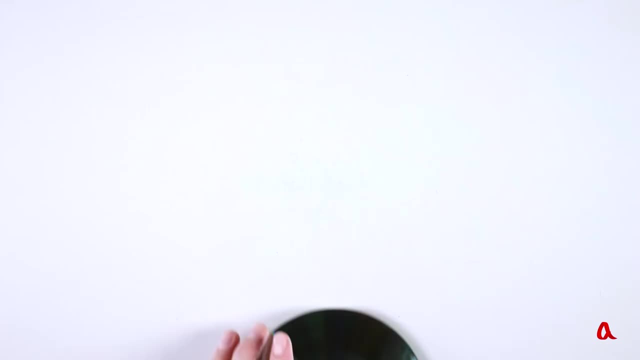 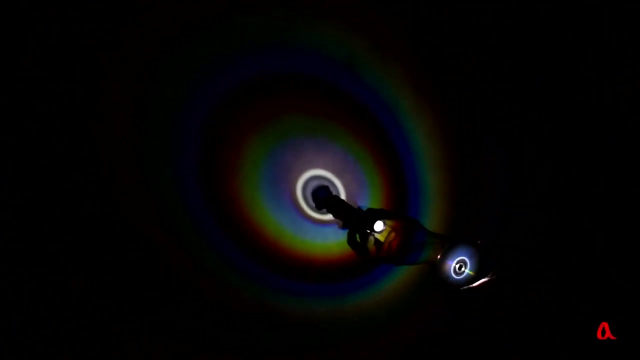 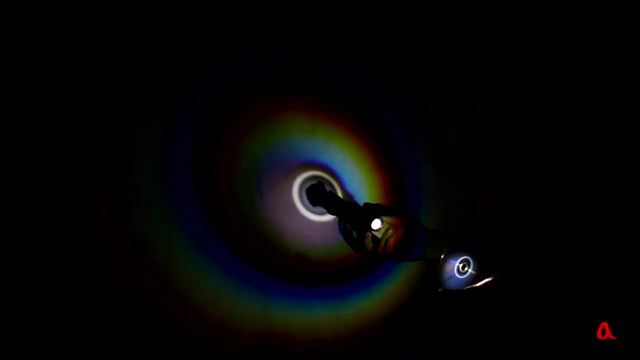 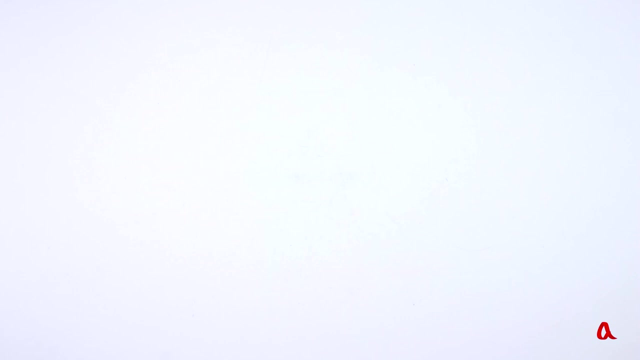 Let us direct a flashlight onto a CD and see what bright colors of the rainbow we obtain as a result. But how does white light decompose into a spectrum? in this case, After all, there is no refraction, like in a prism. Where do rainbow colors come from?